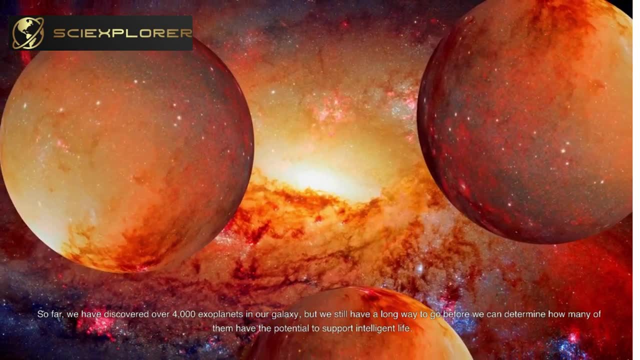 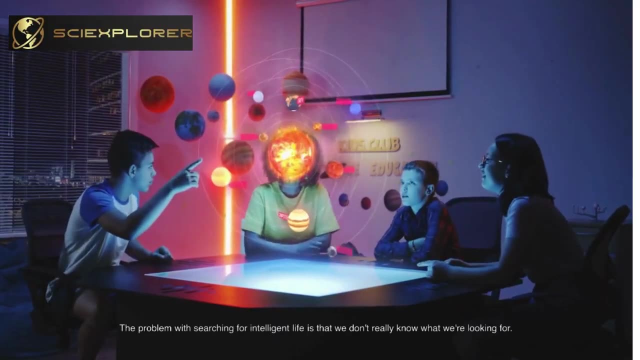 exoplanets in our galaxy, but we still have a long way to go before we can determine how many of them have the potential to support intelligent life. The problem with searching for intelligent life is that we don't really know what we're looking for. We assume that intelligent life 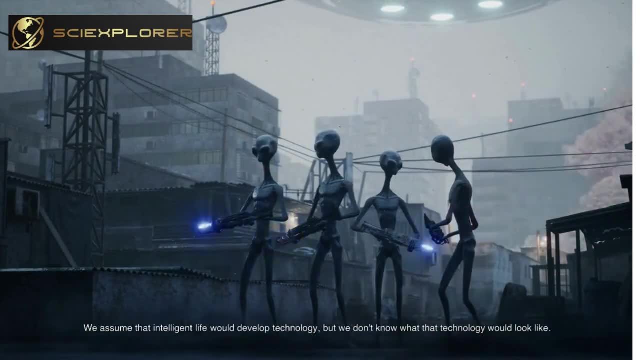 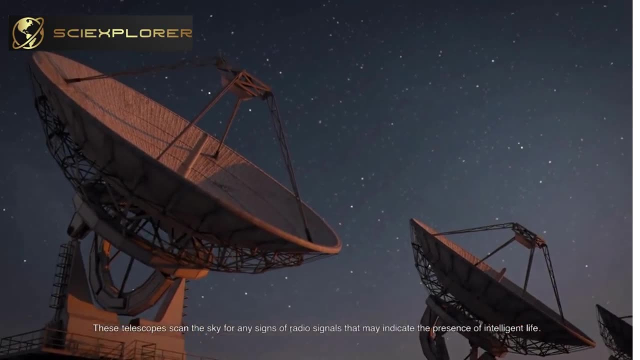 would develop technology, but we don't know what that technology would look like. One method that scientists use to search for intelligent life is through the use of radio telescopes. These telescopes scan the sky for any signs of radio signals that may indicate the presence of 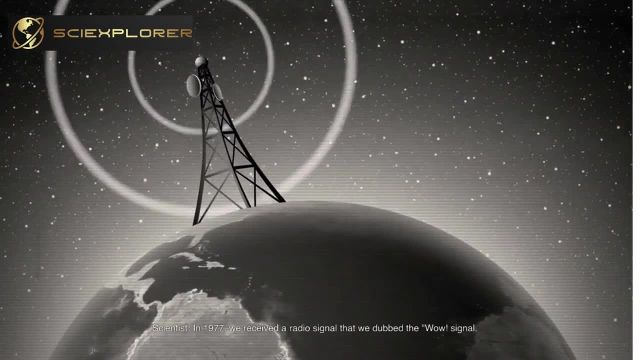 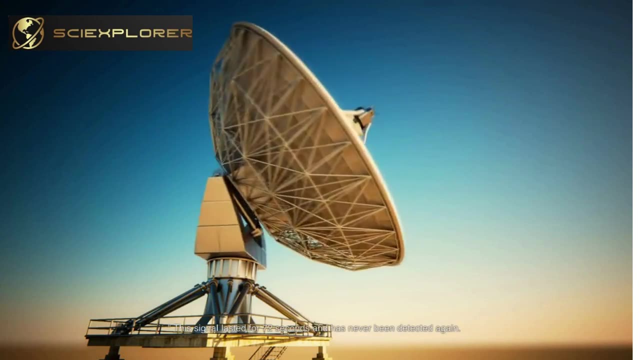 intelligent life Scientist In 1977, we received a radio signal that we dubbed the Wow Signal. This signal lasted for 72 seconds and has never been detected again, While we can't say for sure that it was a signal from an intelligent alien species. 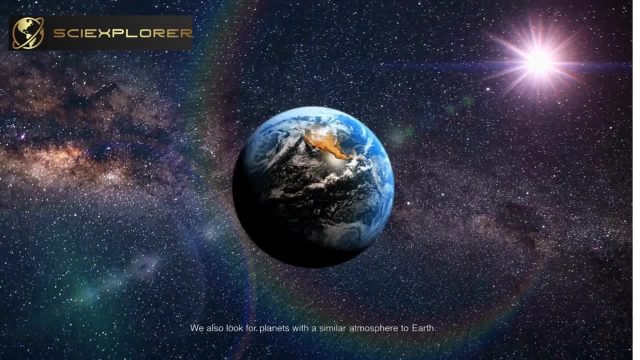 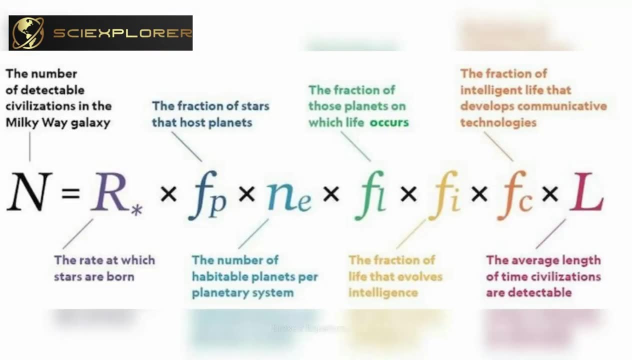 it remains one of the best pieces of evidence we have. We also look for planets with a similar atmosphere to Earth. This can be an indication that the planet has the potential to support life as we know it. Drake's Equation. This equation is a way of estimating the number. 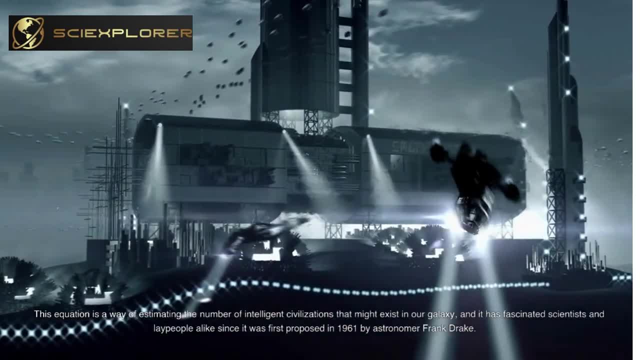 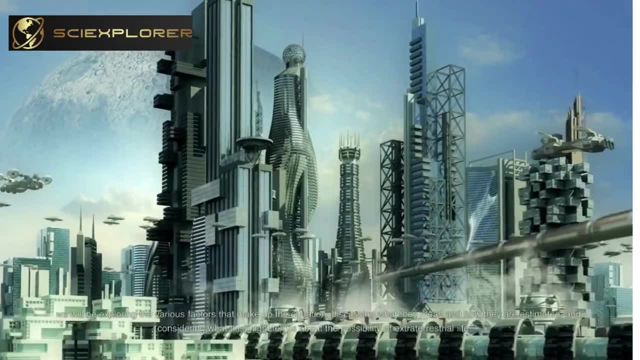 of intelligent civilizations that might exist in our galaxy, and it has fascinated scientists and laypeople alike since it was first proposed in 1961 by astronomer Frank Drake. We will be exploring the various signals that we have. We will also look for planets with a similar atmosphere to Earth. 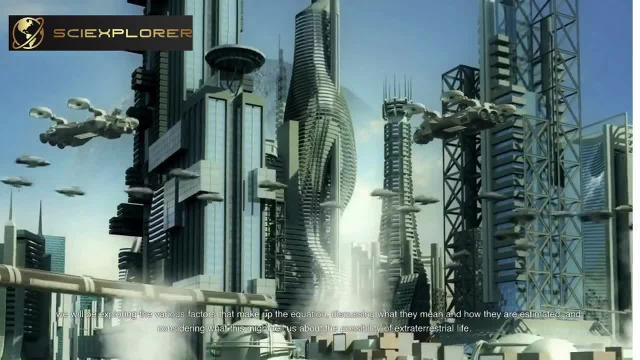 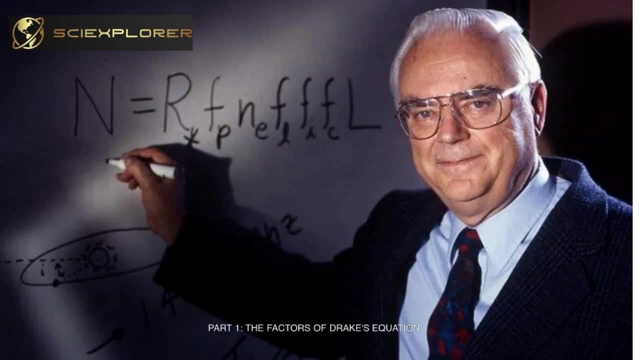 Let's take a look at these factors that make up the equation, discussing what they mean and how they are estimated, and considering what this might tell us about the possibility of extraterrestrial life. Part 1. The factors of Drake's Equation. Drake's Equation is a mathematical formula that 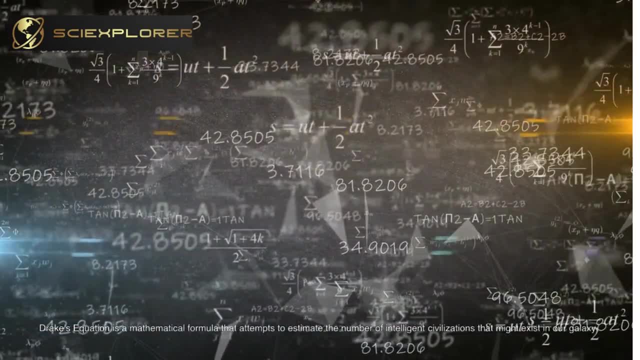 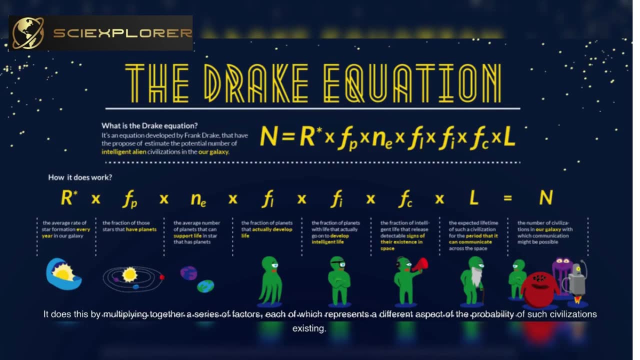 attempts to estimate the number of intelligent civilizations that might exist in our galaxy. It does this by multiplying together a series of factors, each of which represents a different aspect of the probability of such civilizations existing. Let's take a look at these factors in turn. The rate of starvation is the number of stars that exist in our galaxy. The rate of starvation 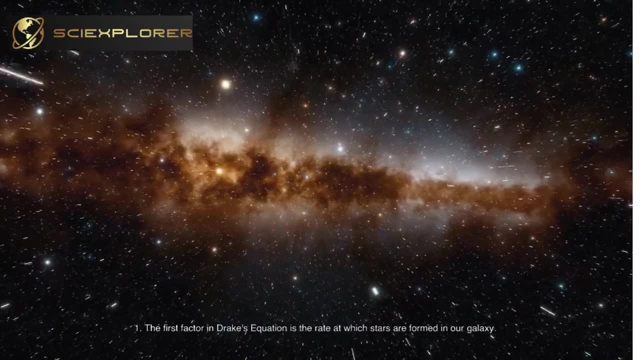 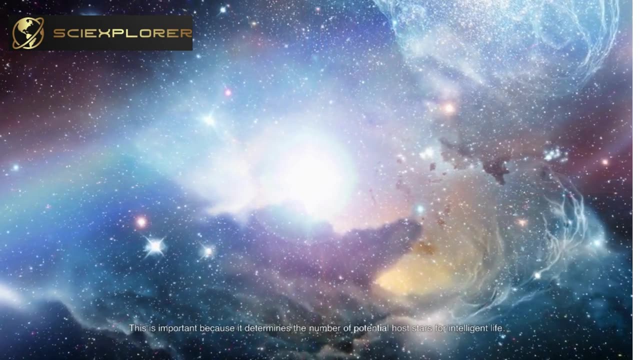 is the star formation. 1. The first factor in Drake's Equation is the rate at which stars are formed in our galaxy. This is important because it determines the number of potential host stars for intelligent life. The current estimate is that around 7 new stars are formed in our galaxy. 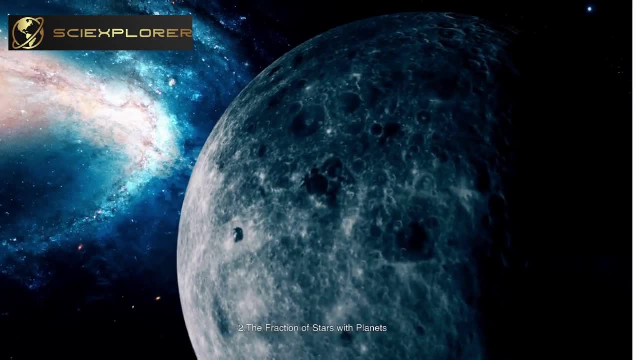 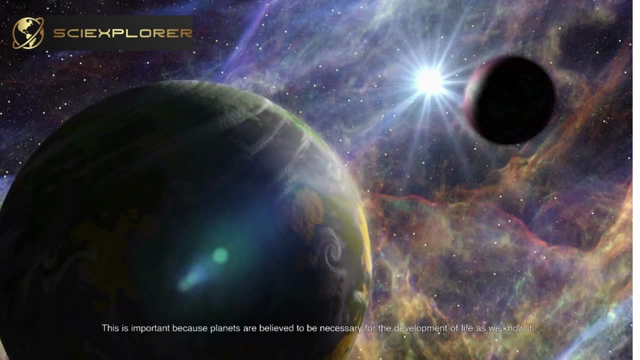 every year. 2. The fraction of stars with planets. The second factor is the fraction of stars that have planets. This is important because planets are believed to be necessary for the development of life as we know it. Recent studies suggest that around 50% of stars are formed in our galaxy. 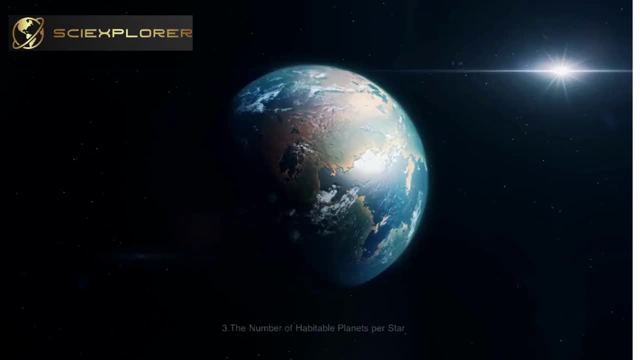 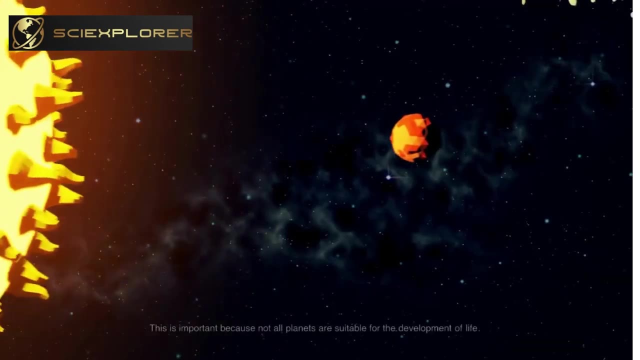 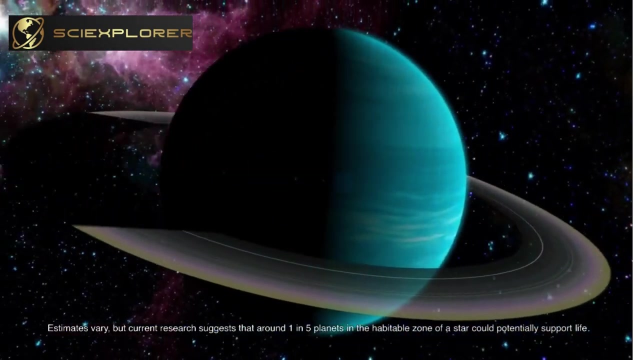 3. The number of habitable planets per star. The third factor is the number of habitable planets per star. This is important because not all planets are suitable for the development of life. Estimates vary, but current research suggests that around 1 in 5 planets in the habitable 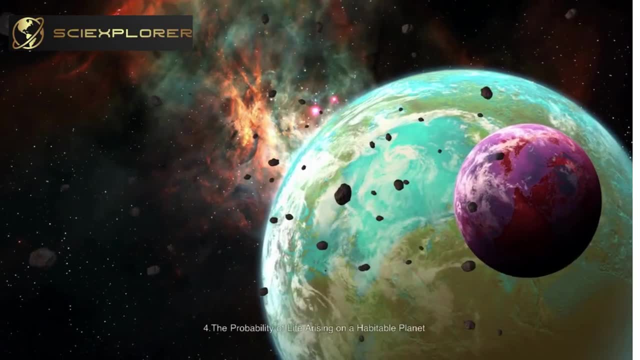 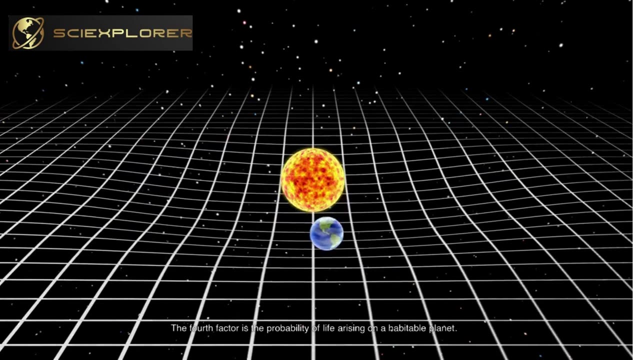 zone of a star could potentially support life. 4. The probability of life arising on a habitable planet. The fourth factor is the probability of life arising on a habitable planet. This is important because, even if a planet is in the habitable zone and has the necessary 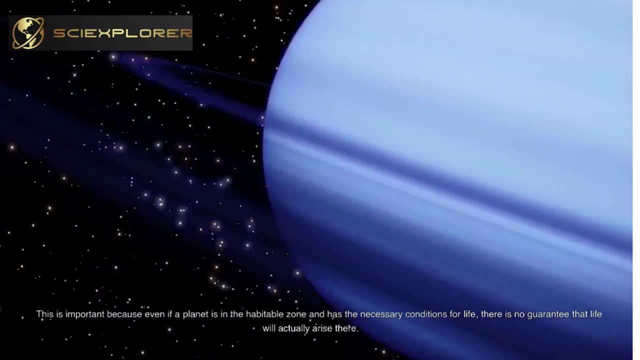 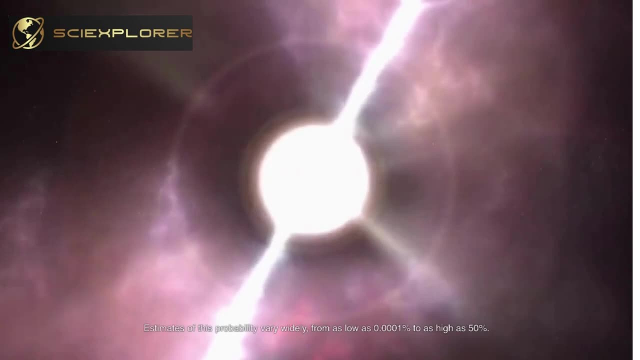 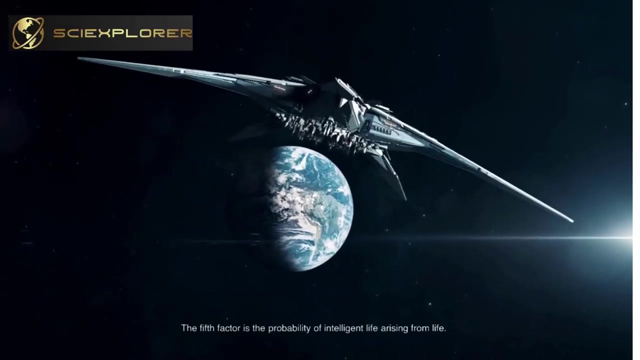 conditions for life, there is no guarantee that life will actually arise there. Estimates of this probability vary widely, from as low as 0.0001% to as high as 50%. 5. The probability of intelligent life arising from life. The fifth factor is the probability of intelligent life arising from life. 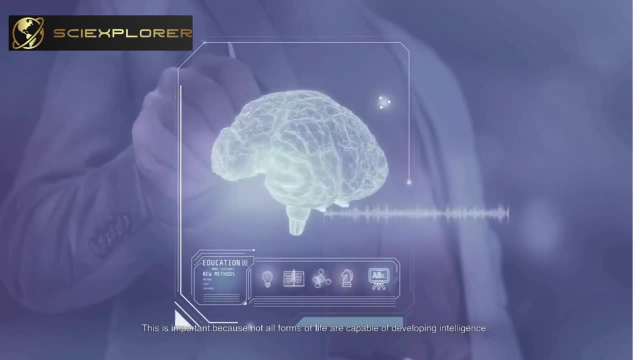 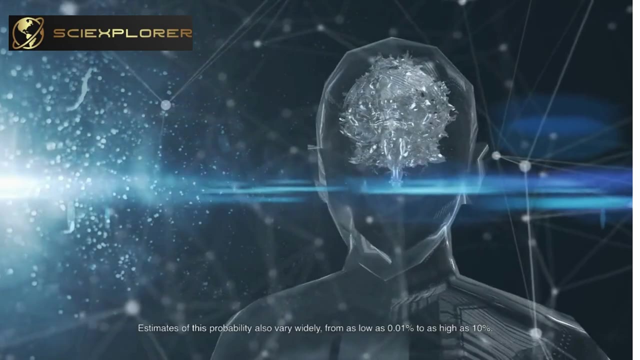 This is important because not all forms of life are capable of developing intelligence. Estimates of this probability also vary widely, from as low as 0.001% to as high as 10%. 6. The length of time a civilization can communicate. The final factor is the length. 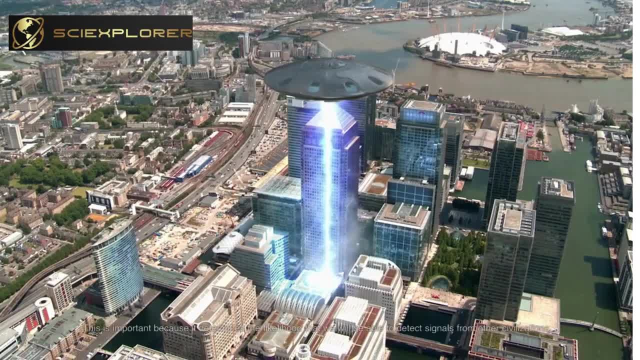 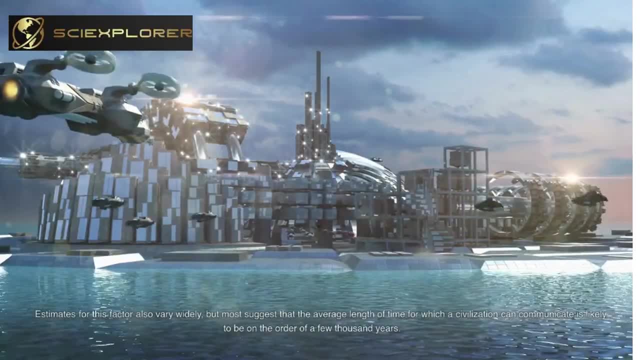 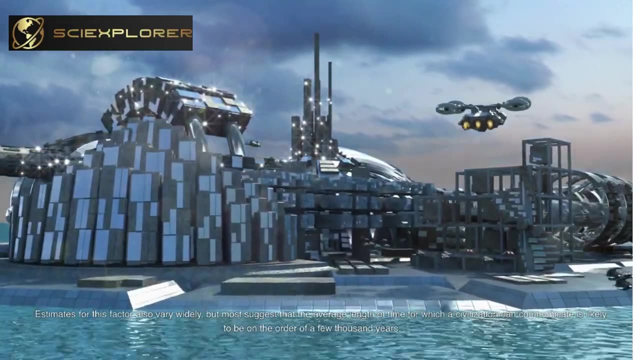 of time that a civilization is capable of communicating. This is important because it determines the likelihood that we will be able to detect signals from other civilizations. Estimates for this factor also vary widely, but most suggest that the average length of time for which a civilization can communicate is likely to be on the order of a few thousand years. 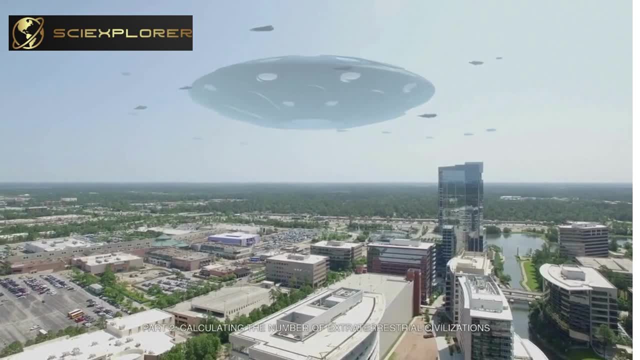 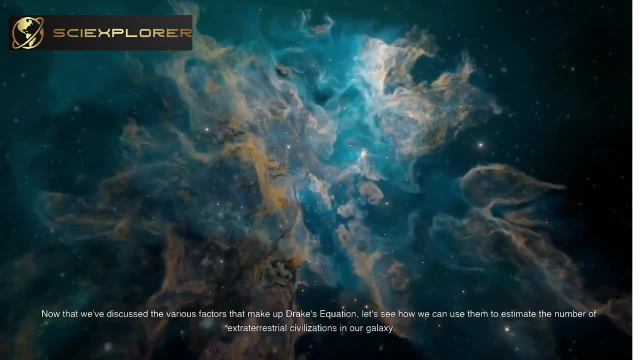 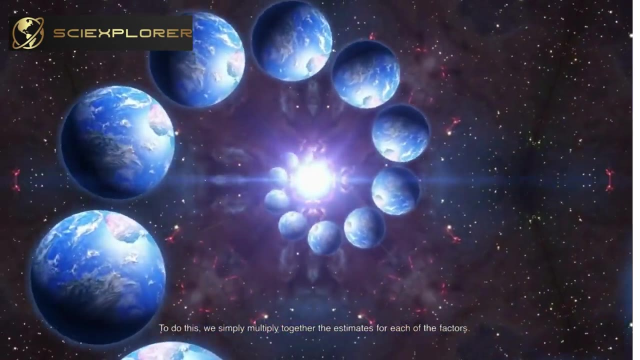 Part 2. Calculating the number of extraterrestrial civilizations. Now that we've discussed the various factors that make up Drake's equation, let's see how we can use them to estimate the number of extraterrestrial civilizations in our galaxy. To do this, we simply multiply together the estimates for each of the factors, Using the 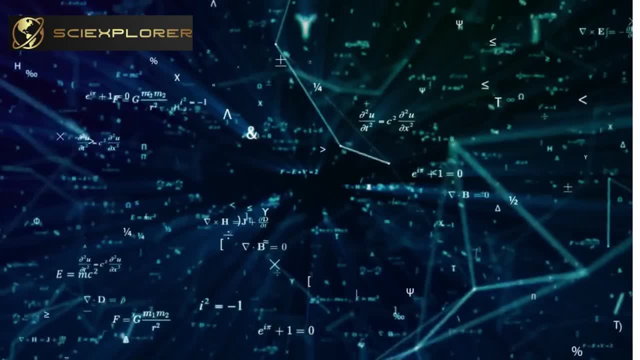 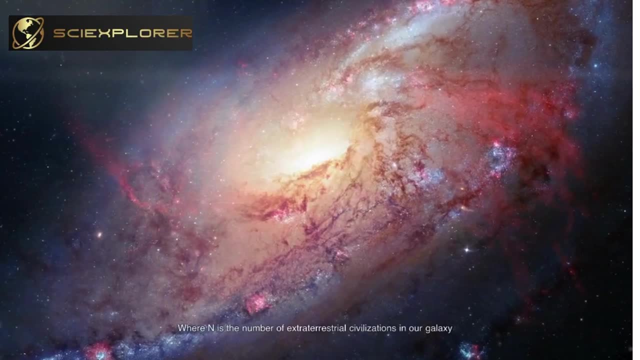 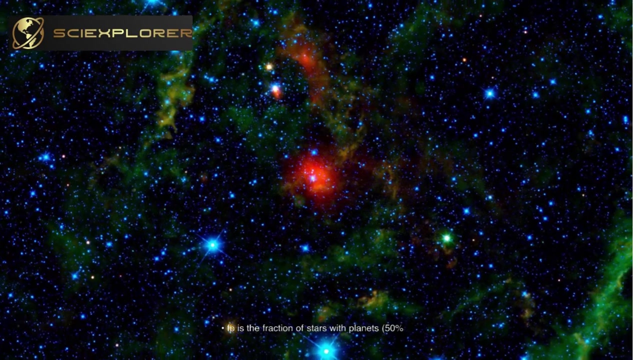 estimates we discussed earlier, we get the following calculation: n equals r, x, f, p, x, ne, x, f, l, x, phi, x, f, c, x, l, Where n is the number of extraterrestrial civilizations in our galaxy, r is the rate of star formation- 7 stars per year. f, p is the fraction of stars with 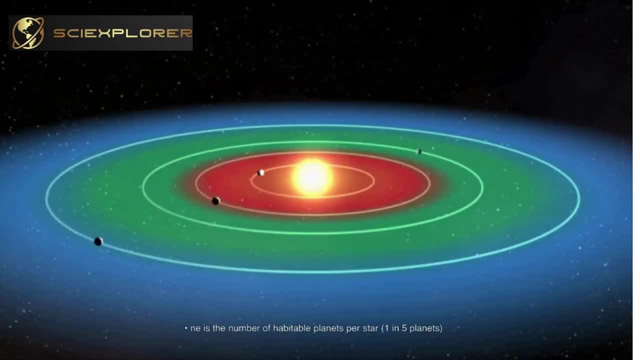 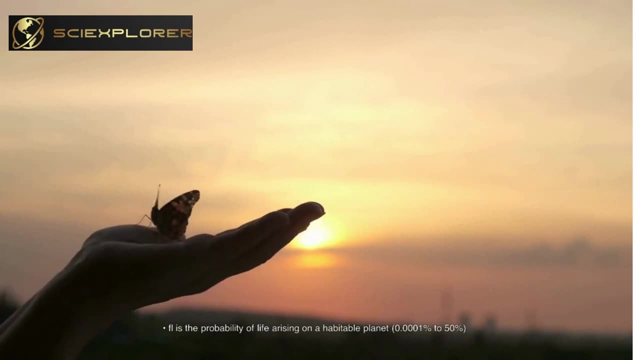 planets. 50%. ne is the number of habitable planets per star. 1 in 5 planets. f? l is the probability of life arising on a habitable planet: 0.0001% to 50%. phi is the probability. 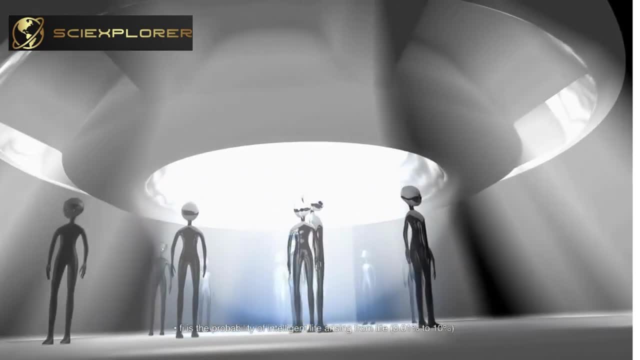 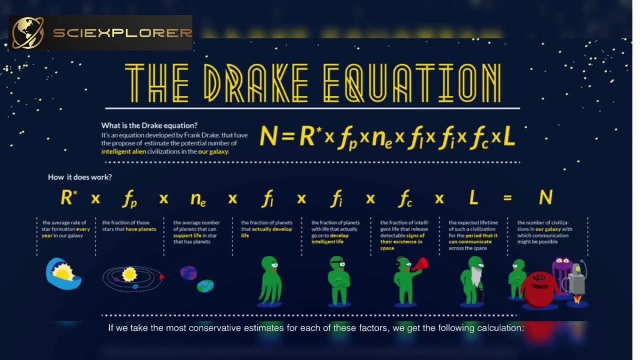 of intelligent life arising from life: 0.01% to 10%. f? c is the fraction of civilizations that can communicate. f? c is the probability of intelligent life arising from life: 0.01% to 10%- A few thousand years, If we take the most conservative estimates for each of these. 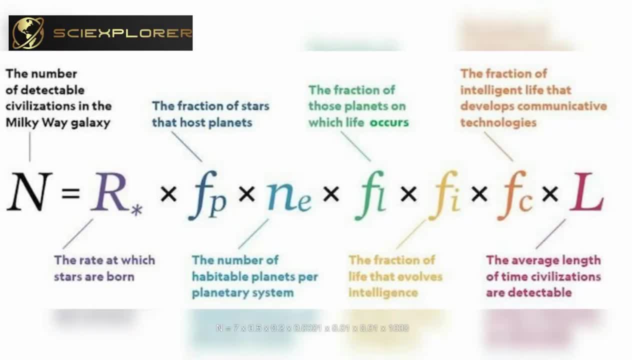 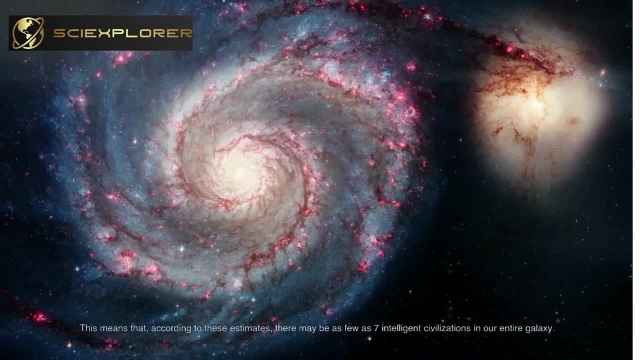 factors, we get the following calculation: n equals 7 by 0.5, by 0.2, by 0.0001, by 0.01, by 0.01 x 1000.. n equals 0.0000007.. This means that, according to these estimates, there may be as: 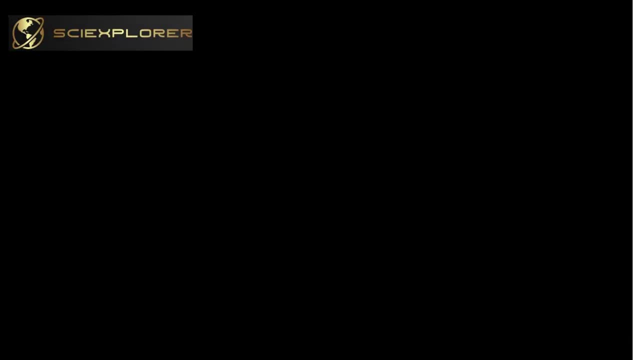 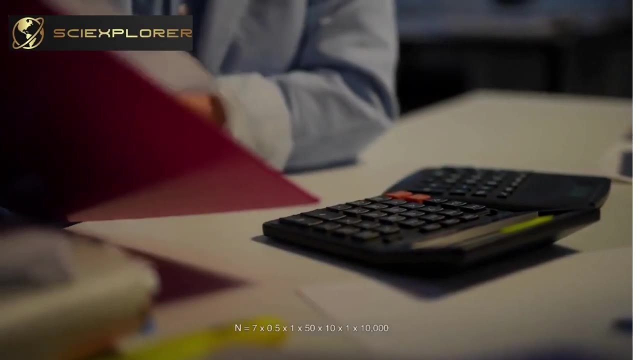 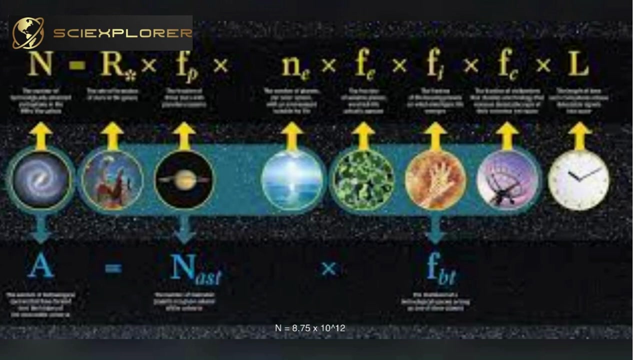 few as 7 intelligent civilizations in our entire galaxy. However, if we take the more optimistic estimates for each factor, we get a much larger number. n equals 7 by 0.5 x 1 by 50 by 10 by 1 by 10,000.. n equals 8.75 x 10 to the power of 12.. This means that, according to these 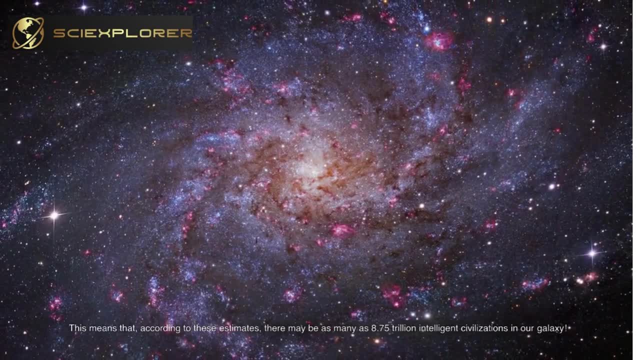 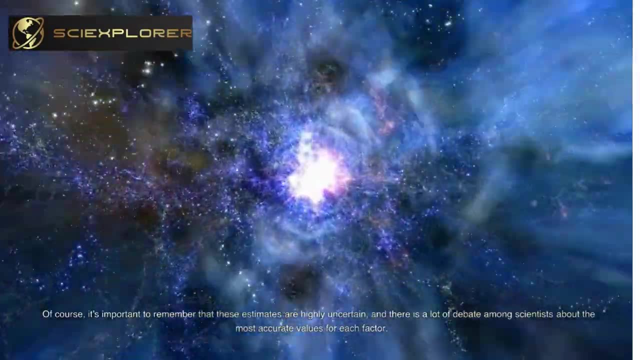 estimates, there may be as many as 8.75 trillion intelligent civilizations in our galaxy. Of course, it's important to remember that these estimates are highly uncertain and there is a lot of debate among scientists about the most accurate values for each factor. However, 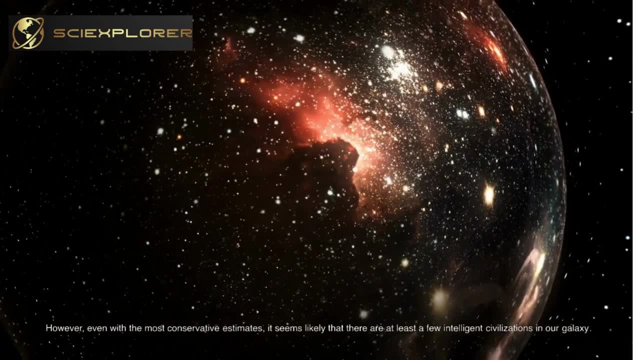 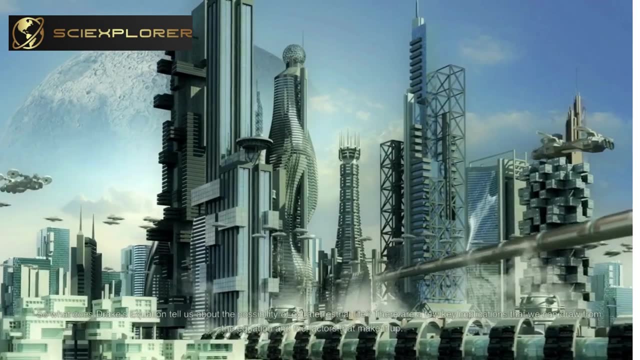 even with the most conservative estimates, it seems likely that there are at least a few intelligent civilizations in our galaxy. Part 3. Implications of Drake's Equation. So what does Drake's Equation tell us about the possibility of extraterrestrial life? 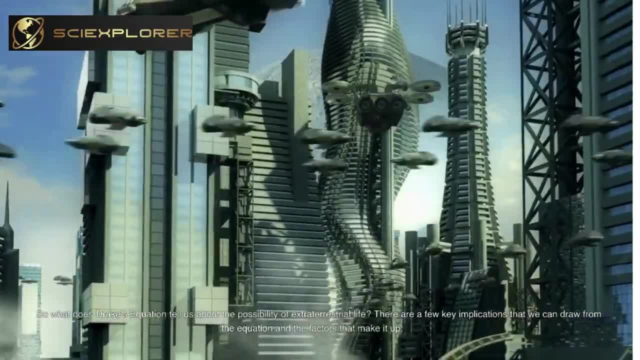 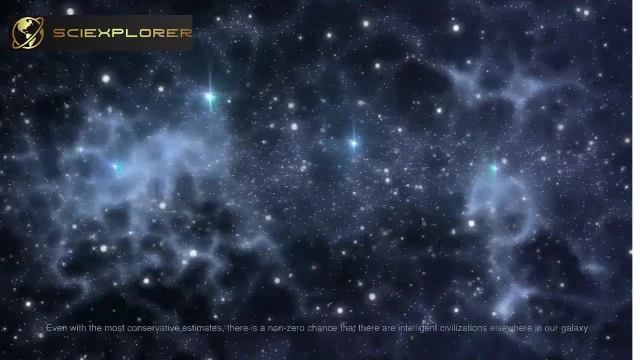 There are a few key implications that we can draw from the equation and the factors that make it up. Firstly, the equation tells us that the existence of extraterrestrial life is not impossible. Even with the most conservative estimates, there is a non-zero chance that there are.